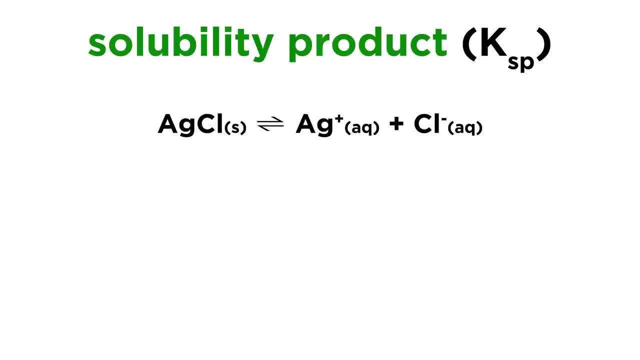 Just as with any other type of equilibrium, there must be an equilibrium constant to describe it, and that's the solubility product. As we might guess, this will simply be equal to the product of the two ion concentrations in solution, each raised to the power of their stoichiometric coefficients, which, in this 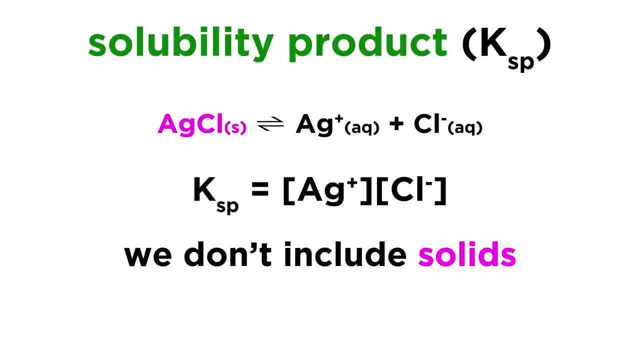 case is simply one and one. We do not include the solid itself in this expression, as we do not include solids in equilibrium expressions. The smaller the constant, the fewer the ions that will be present in solution and therefore the less soluble the substance must be. 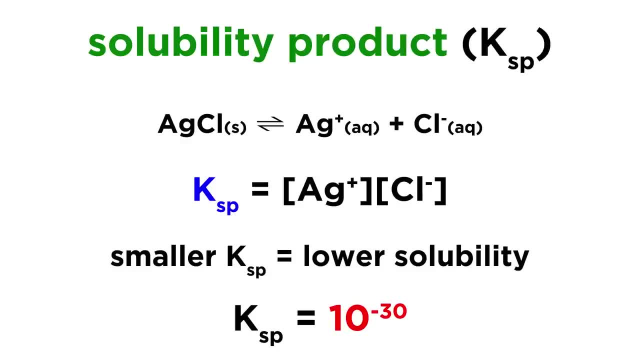 And compounds that are extremely water-insoluble will have Ksp values on the order of ten to the negative, thirty, negative fifty or even smaller. Let's make sure we can write these solubility products. Take something like calcium carbonate First. we must write out the complete equilibrium. 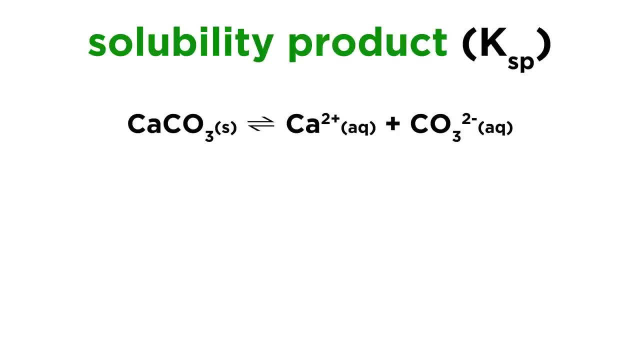 Upon dissociating, this will form a calcium ion and a carbonate ion. Therefore, the solubility product will be equal to the product of these two ion concentrations. If we have something like magnesium hydroxide, it's the same thing, except that dissociation. 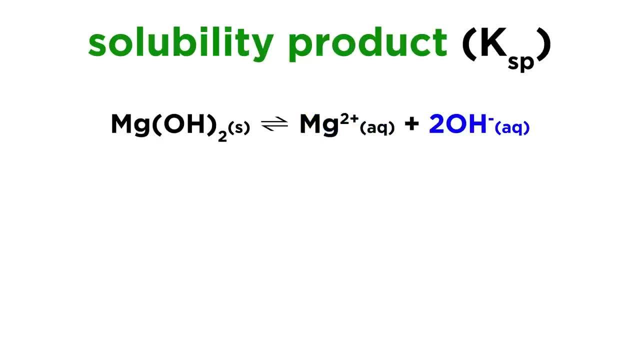 produces one magnesium ion and two hydroxides. This means that the hydrogen ion concentration will be squared in the solubility product expression. We can even do this for something more complicated, like apatite, which is a mineral. This will dissociate into five calcium ions, three phosphate ions and a hydroxide ion. 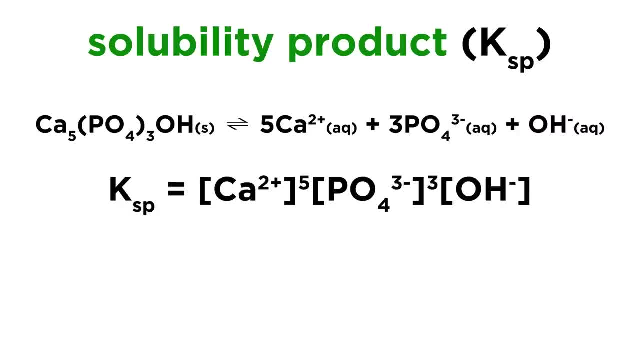 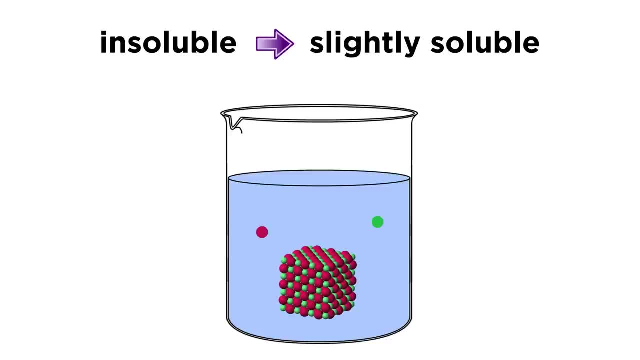 so the solubility product expression will look like this: In this way, a number of ions will be dissociated into one calcium ion and one hydroxide ion. The number of ionic compounds that we previously deemed insoluble should actually be categorized. 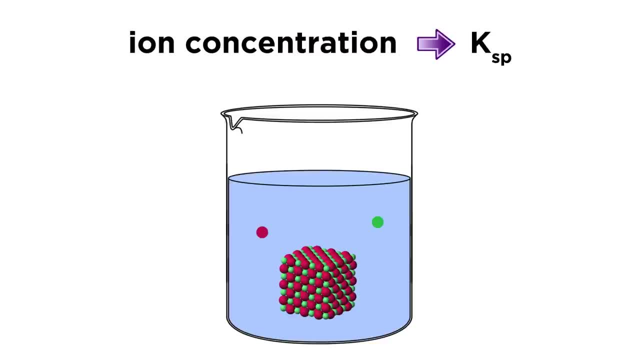 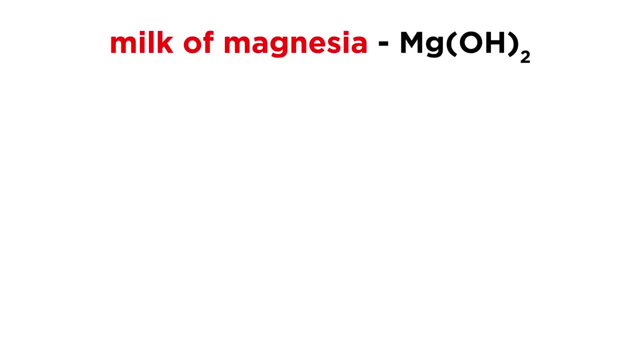 as slightly soluble. If we have a way of measuring ion concentrations in solution, we can calculate the Ksp value for a given substance. Let's say we have a saturated solution of milk of magnesia which is magnesium hydroxide. This is slightly soluble and dissolves according to the following equilibrium: 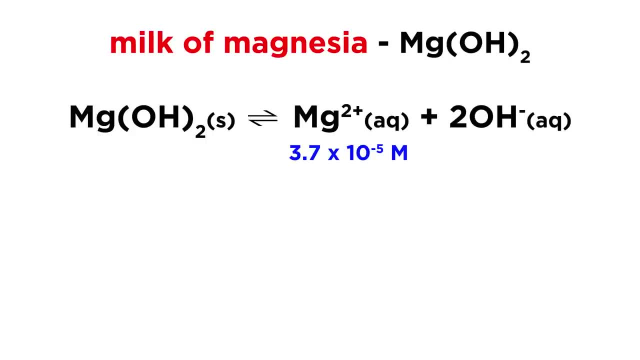 This is slightly soluble and dissolves according to the following equilibrium: This is slightly soluble and dissolves according to the following equilibrium: What will be the solubility product for magnesium hydroxide? First, let's write the Ksp expression for this substance which we derived earlier. 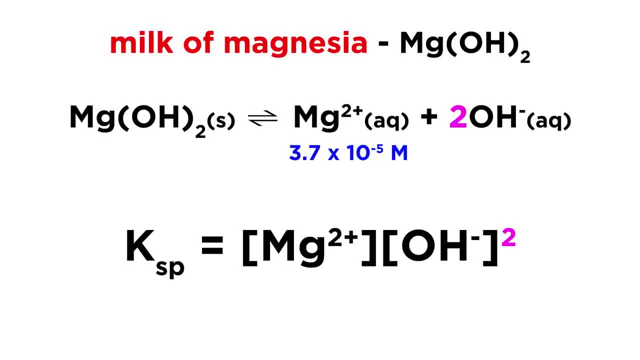 Notice that hydroxide concentration is squared due to the coefficient in the equilibrium. Now, if this is the concentration of the magnesium ion, then the hydroxide ion concentration must be precisely double, Since there are two hydroxide ions for every magnesium ion in this substance. so all we 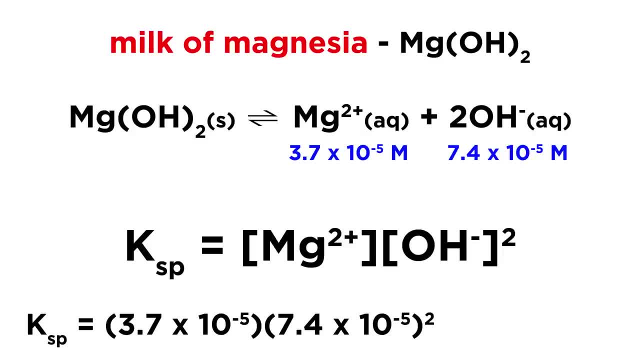 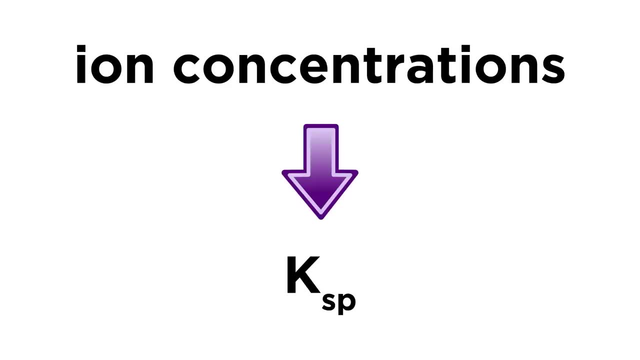 need to do is plug these two concentrations into the expression evaluate and we will get 2.0 times 10 to the negative 13 for Ksp, which will be a unitless constant, just like other equilibrium constants. We can also go the other way around and predict the concentrations of ions that will result. 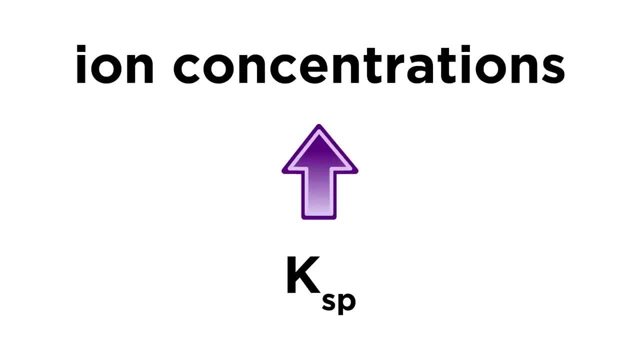 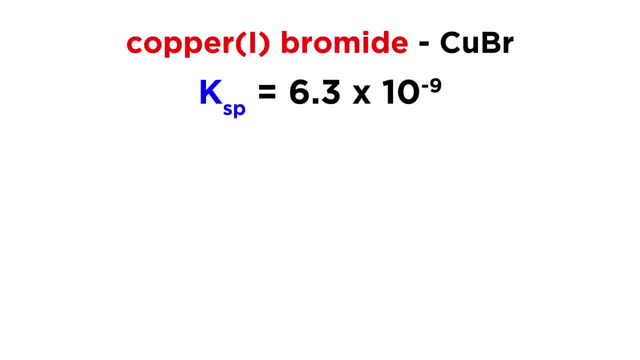 in solution. Let's say we place copper bromide, which has a Ksp of 6.3 times 10 to the negative 9, in aqueous solution, which will then generate copper ions and bromide ions to some extent. What will be the molar solubility of this substance, meaning how many moles per liter? 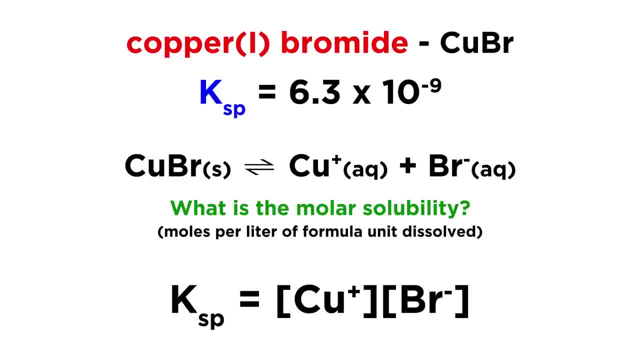 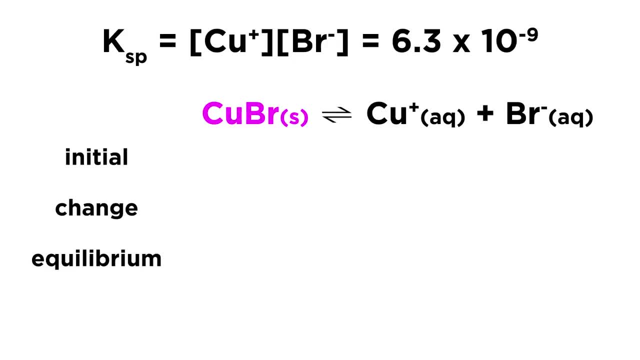 of the formula unit will dissolve. To find this, we can write the solubility product expression and use this to construct a simple ice chart. In this we will not list any values for copper bromide, as this is a solid. 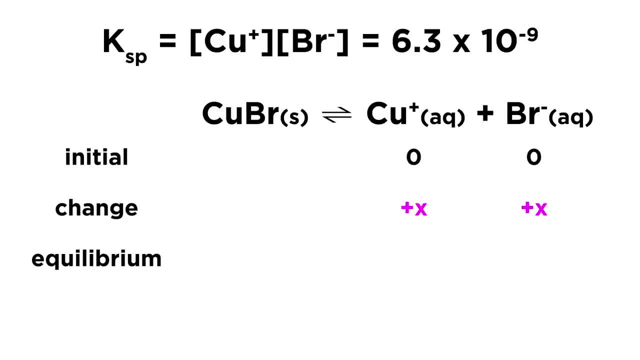 The ions themselves will start at zero. the change will be X because of the one to one to one ratio, and this means that the equilibrium concentrations of the ions will also be equal to X. Therefore, the Ksp will be equal to X squared and X will be 7.9 times 10 to the negative. 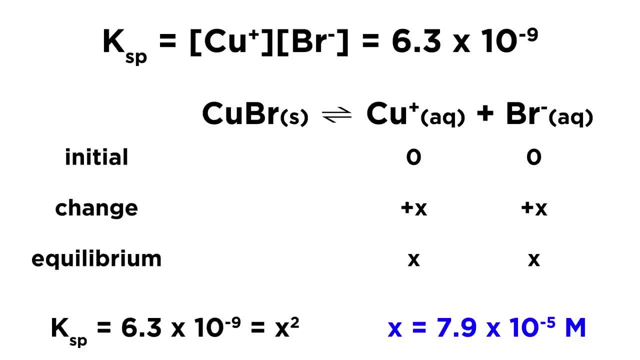 five moles per liter. This is the molar solubility of copper bromide, which in this case is simply the concentration of copper ions and bromide ions in solution at equilibrium. This can be a little trickier if the Ksp equation involves exponents, but the process is essentially. 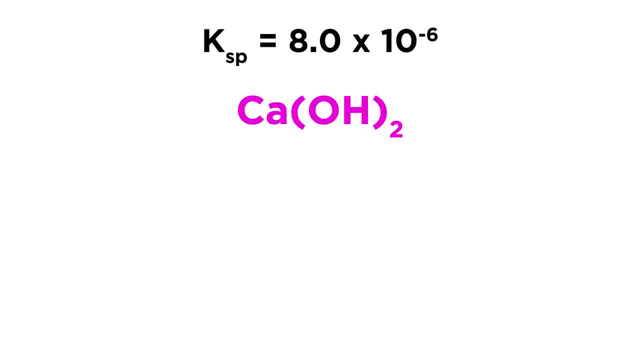 the same. Let's look at calcium hydroxide, which has a Ksp of 8.0 times 10 to the negative six. Say we place this in aqueous solution, which will produce some calcium ions and hydroxide ions. 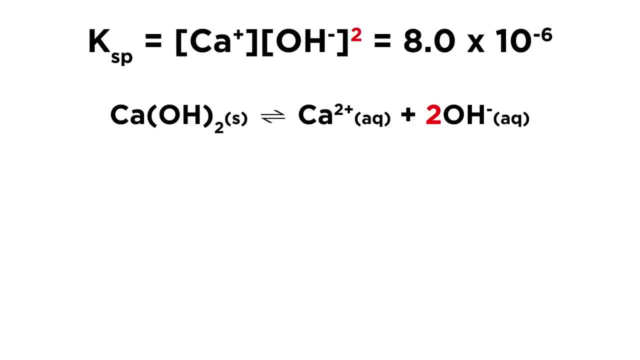 Again, let's write the Ksp expression, noticing that the hydroxide concentration must be squared, as there will be two hydroxide ions for every formula unit of calcium hydroxide that dissolves. Then when we make the ice chart, we will notice that again, the initial concentration of each 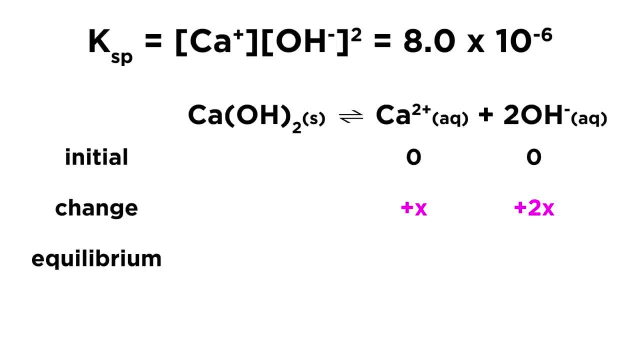 ion will be zero, but the change will be X and two X respectively, due to the stoichiometry of the equation, and the equilibrium concentrations will also be X and two X. Putting these into the Ksp expression, we get that the Ksp will be equal to four X cubed. 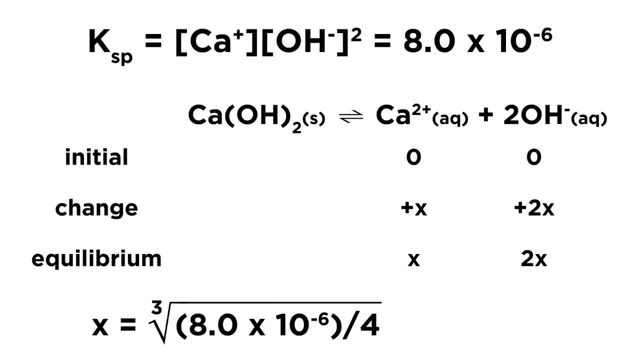 Now solving for X. we divide by four and then take the cube root, leaving us with one point three times ten to the negative two for X, which will therefore be the molar solubility, which we can interpret as the solubility of the solid expressed in moles per liter, or 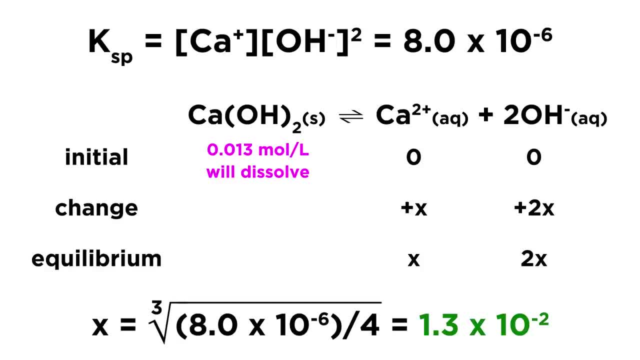 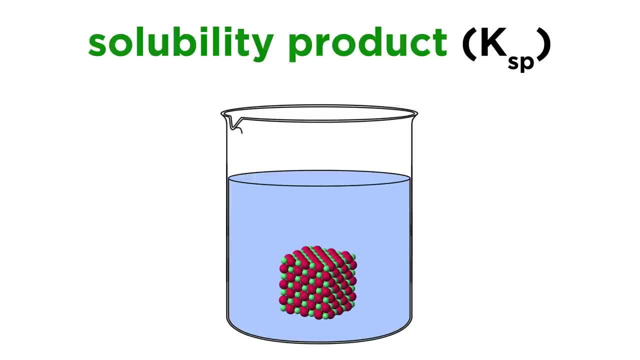 the moles of the solid that will dissolve per liter of water. So now that we've looked at the Ksp expression, let's look at the Ksp expression. We get that the Ksp will be equal to four X cubed. Now we've learned a bit about the solubility product. it's time to learn a few applications. 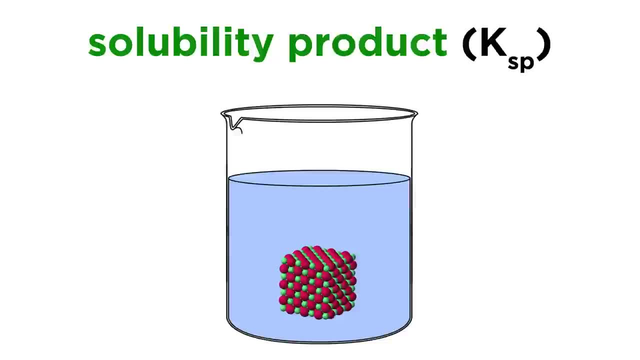 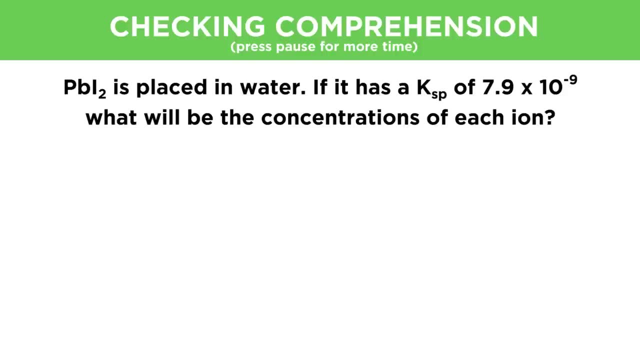 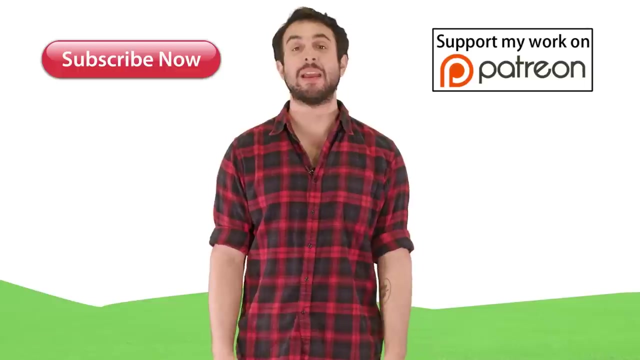 of this concept, But first let's check comprehension. Thanks for watching, guys. Subscribe to my channel for more tutorials, support me on patreon so I can keep making content and, as always, feel free to email me professordaveexplains at gmail dot com. 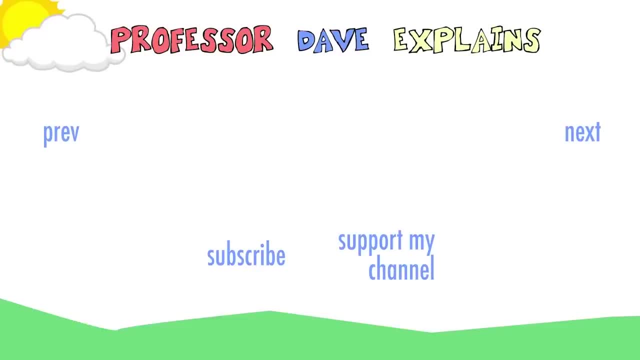 I'll see you in the next one.